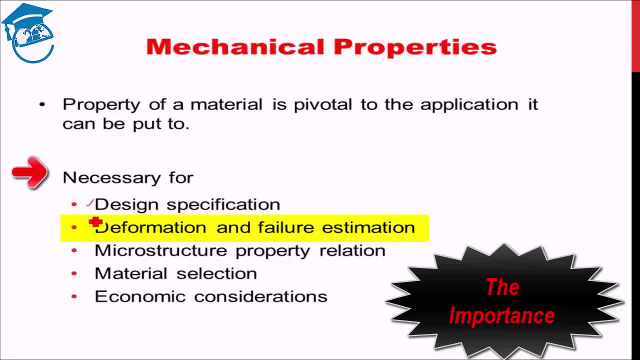 deformation mechanisms And, as a result of that, what are the possible failure mechanisms that can be present in a body And we can estimate the lifetime of a material for a particular application? 1 when the failure is going to occur and this knowledge of failure being able to. 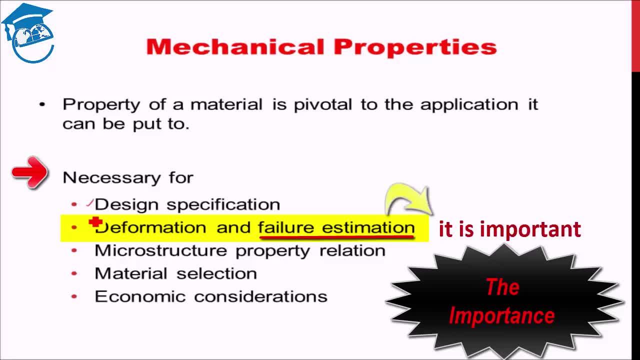 predict that beforehand is very, very important, because the engineering materials are used in different scenarios, from bridges to buildings, to aircrafts, to automobiles, where any failure can be the difference between life and death, and the knowledge beforehand of when a possible failure can occur will be very, very handy. Therefore, the knowledge of mechanical 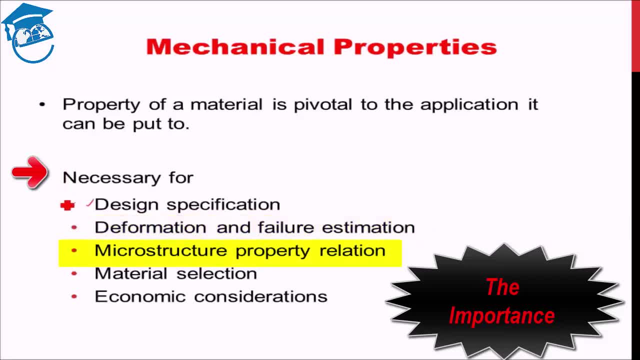 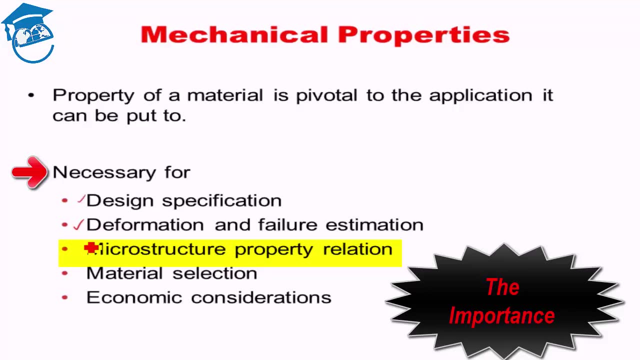 properties is quite important. The knowledge of mechanical properties also lets you find the relation between microstructure and property Right. so the idea is different. microstructure has different kind of property behaviors- Right. so the idea is different. microstructure has different kind of property behaviors. 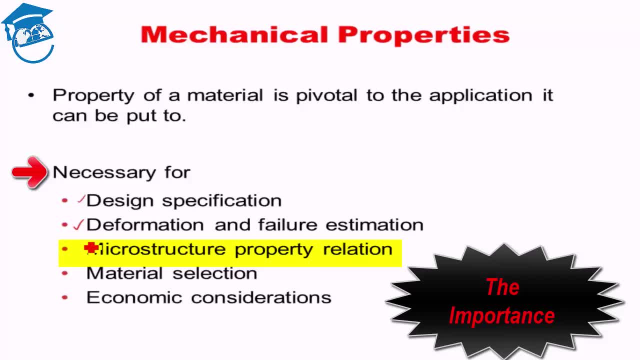 So only when you know what are the mechanical properties that needs to be identified in a given material, you study those properties for different microstructures. Now, once you know the property values for different microstructure, you can pinpoint that okay, I need this kind of microstructure or this kind of material for a particular. 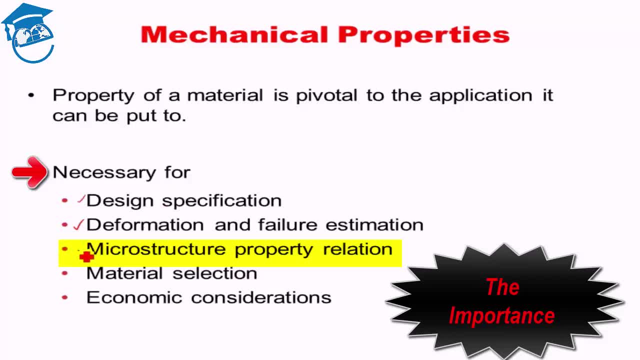 application. Therein also comes your material selection. right, Microstructure as well as what is the metal, whether it is iron, whether you are going for steel, whether you are going for aluminium. the material selection will also depend on what are the mechanical property requirements to be met. 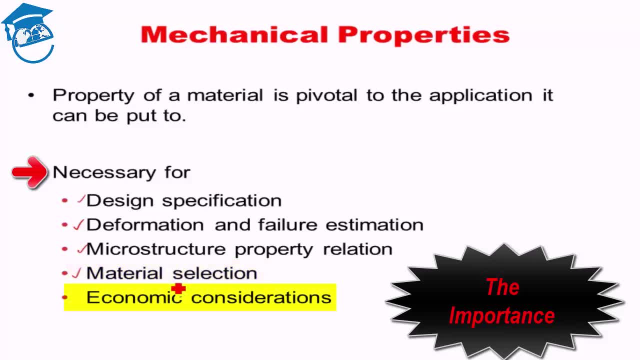 And last but not the least, you can create a very exotic material which has very good strength, very good ductility, It has very nice height, Hardness, impact, resistance and what not. But suppose it is so expensive that it has no practical application. you cannot use it. 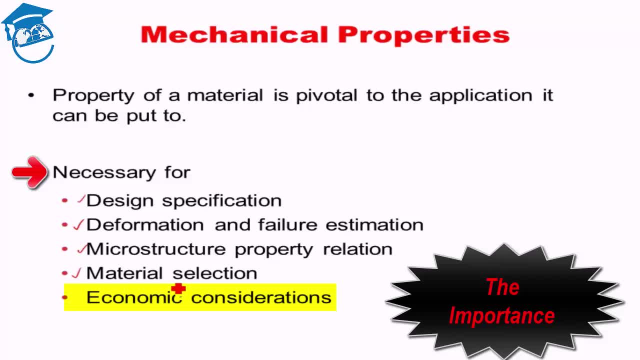 to build bridges. you cannot use it to make new cars. then it's just a showcase. You are not going to bring it into practical application. So, last but not the least, are economic considerations: whether the material which we have is suitable economically for a particular application. 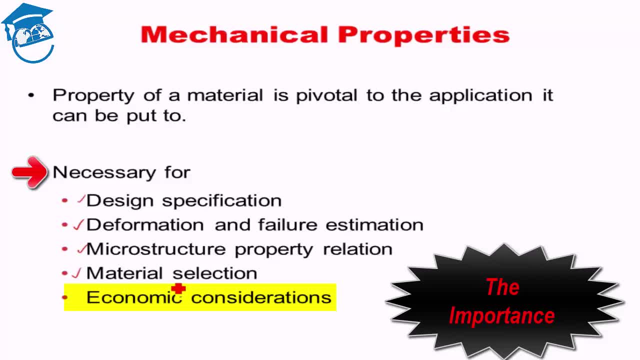 You certainly would like to have a material which has very good properties overall, but you need to select a material which is the most cost effective without compromising with the safety of our requirements. So this kind of gives you a glimpse of why mechanical properties is necessary to be identified. 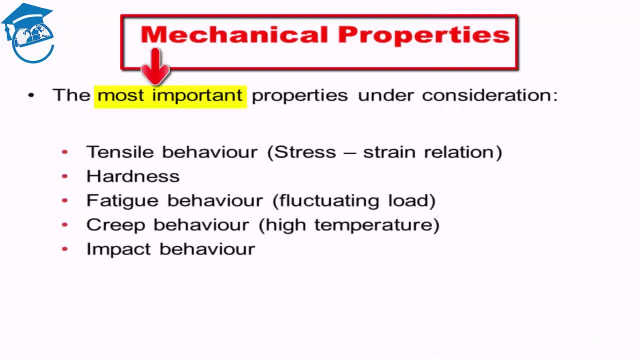 and to be understood. Now, some of the mechanical properties which we will be studying in little details in our unit are the tensile behavior, hardness, fatigue behavior, creep and impact behavior. What are each of them? Tensile behavior basically relates what is the response of the material when you load. 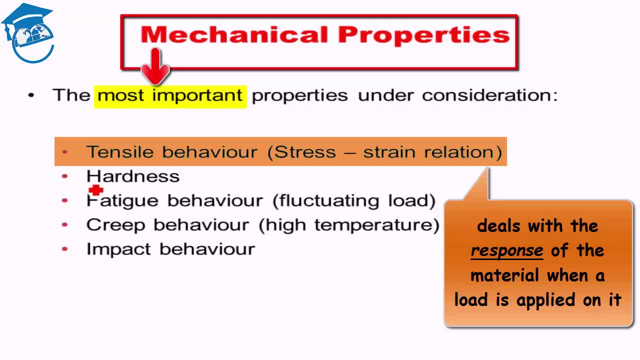 the material. When you apply a load on the material, whether it is tensile or compressive, what is the response that the material is showing? Suppose you have a block. Okay, You have a block, you apply tension. then, for how much load, how much force? what extent? 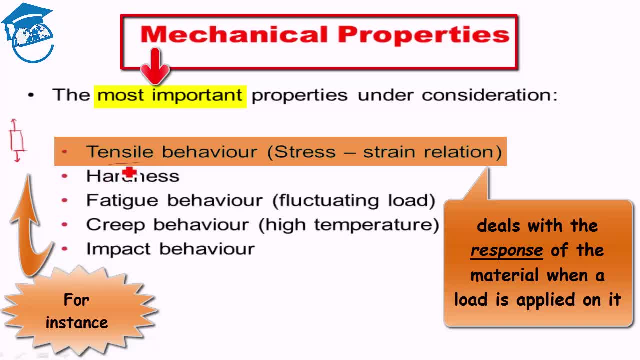 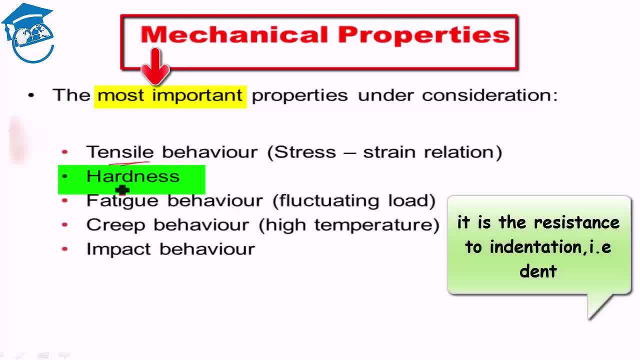 of elongation is taking place. that is what tensile behavior means. Hardness- hardness is basically the resistance to indentation. Suppose you have a load which is being applied. suppose you have a material and a point load of very high magnitude is applied at a particular location. 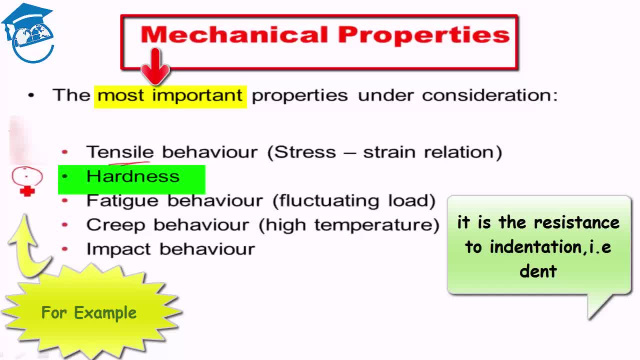 So what is the resistance of the material to that indentation? That is where hardness comes into picture. Fatigue behavior is the behavior of a material under fluctuating load. In this case, what we saw is that the load is constant. You have applied a particular load and you see the response. 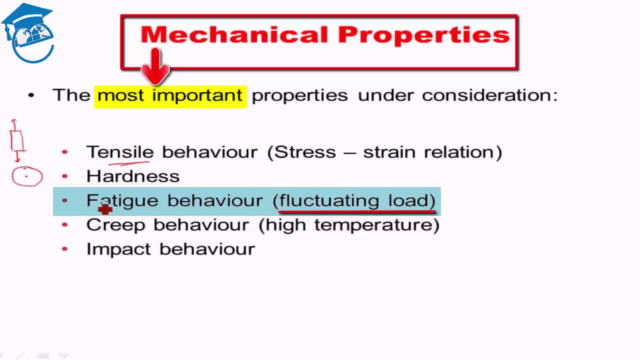 That is the tensile behavior. But suppose you have fluctuating load, For example a bridge. there can be different fluctuating load, Different vehicles, different number of vehicles are passing through it, Different wind velocity is there. So these are fluctuating loads, right? 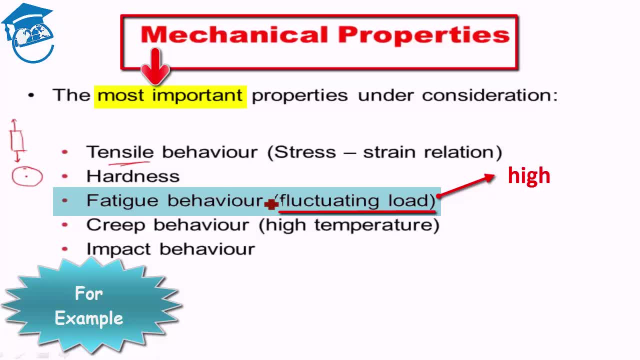 Sometimes the load is quite high, sometimes the load is very nominal. So what is the response of the material to fluctuating load That is studied under the fatigue behavior. Now, what is creep behavior? Creep behavior is basically what is the property of a material at elevated temperature. 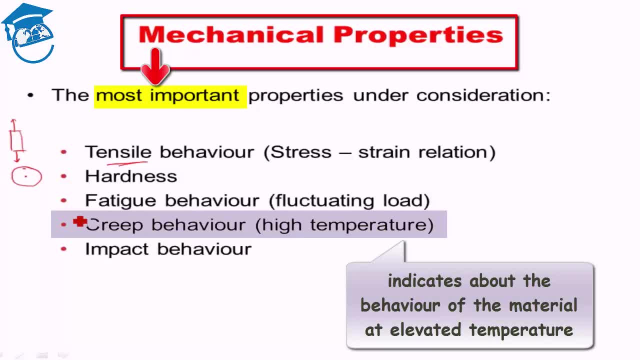 At higher temperature, the material property varies from that at room temperature Or that at lower temperature. So what exactly is the behavior at elevated temperature That is studied under the creep behavior? Impact behavior is basically: you have a material and you provide a load to it in the form of. 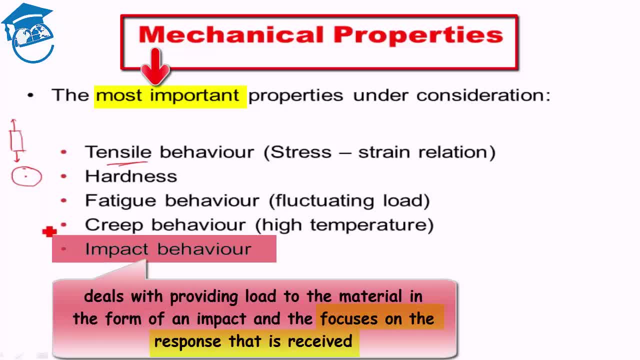 an impact. So what is the response of the material under impact? That is what is studied in impact behavior. This is also- we can think about it- as fracture mechanism. What is the fracture mechanisms of a particular material? So these are broadly the main mechanical properties that we will be studying in this unit. 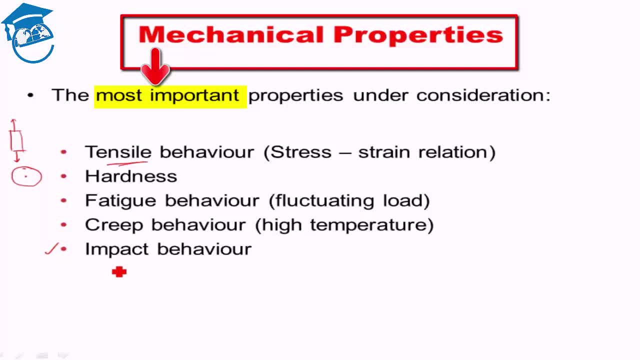 There are many other properties, but these kind of gives you a holistic picture of the most important requirements that are tested by engineers while choosing a material for a particular application. Okay, Now let us start by understanding something. One thing about stress and strain relationship. 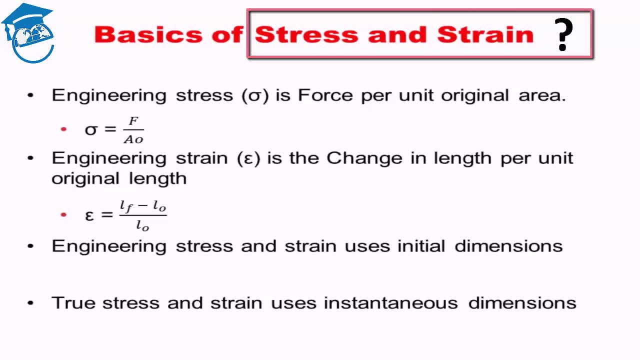 So, to begin with, what is stress and what is strain? There are two types of stress and strain we will be discussing here. One is known as the engineering stress and strain, and the other will be true stress and strain. This slide will mainly deal with engineering stress and strain. 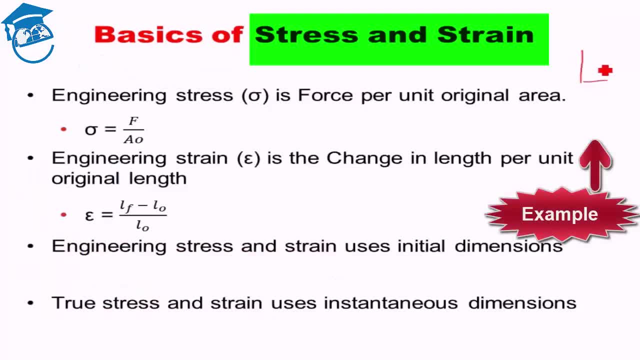 Okay. So suppose we have a block In which I applied a load or a force, F, And the area of cross section of the block, The area of cross section, is A naught. Okay. So when you apply force upward and downward, then the material will try to resist any transformation. 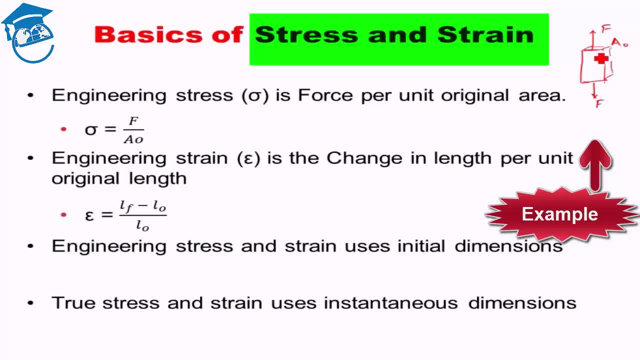 But the material will actually transform. So the engineering stress- Okay, Is force applied per unit area. So force by original area is engineering stress. Engineering stress is denoted by a sigma, Okay, And engineering strain is what is the change in length per unit original length? 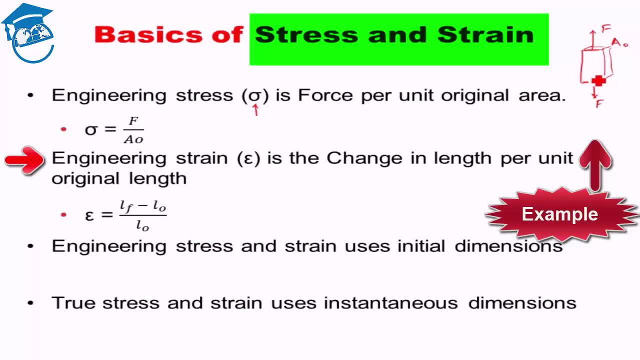 So this applied force will result in a change of length, change of dimension of the body. So how much change of dimension is taking place? That is what strain denotes. Suppose initially it was a length L naught and on application of force, what happens is? 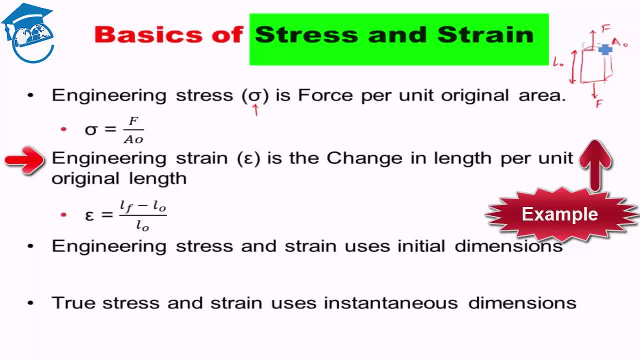 there is an elongation of the body And the final length now becomes LF. So there is a change of length, LF. Okay, of length, delta L is equal to LF minus L naught. This is the change of length, and engineering strain will be change of length per unit. original length. Fine, Now that we know engineering. 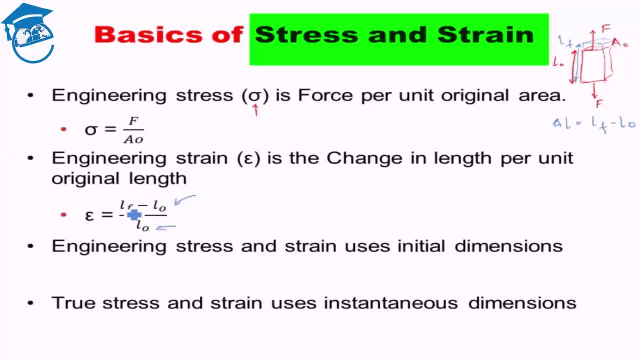 stress and engineering strain. I will give you an idea about what is the difference between engineering stress, engineering strain and true stress, true strain, As we have seen. both for engineering stress and strain, the denominator is the initial dimension. For stress, it was the initial area of cross section. For strain, it was the initial length. But 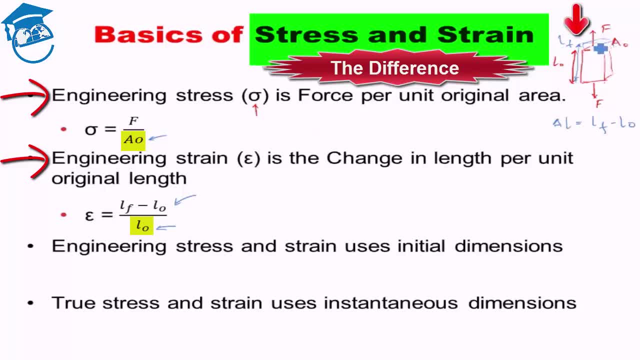 if you think about it, as soon as the dimension starts changing, since the volume needs to be constant, an increase in length will lead to a reduction in area. Right For the volume to be constant, Because volume is equal to length into area. 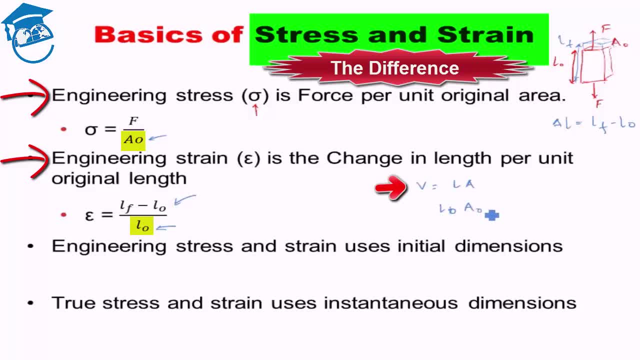 So LF minus LL, L initial into area initial is equal to length final into area final. Now, since L final is more than L initial, area final will be less than area initial. We have not taken into account the instantaneous area till now. That is exactly what true stress and true. 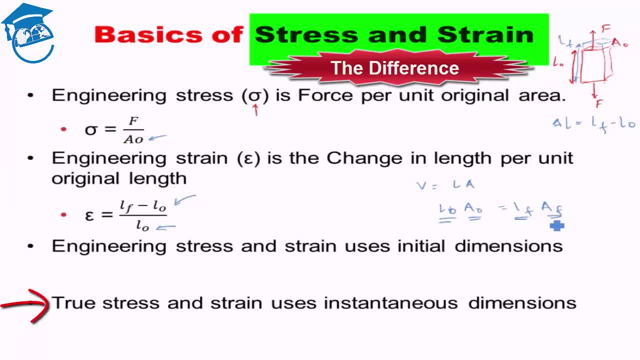 strain does. True stress takes into account the instantaneous area at any time. So true stress is more like F upon L And strain is also dependent on the instantaneous dimensions. So that is the basic difference between engineering stress and true strain. The most of the applications, most of the 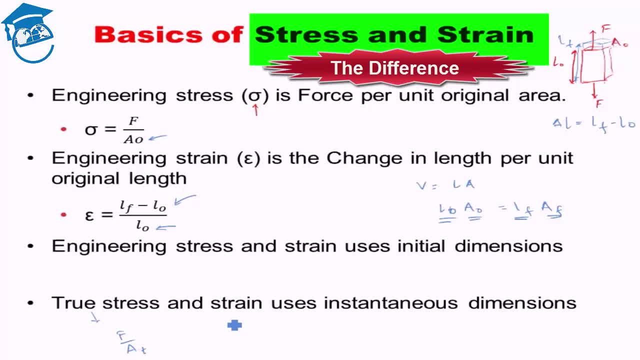 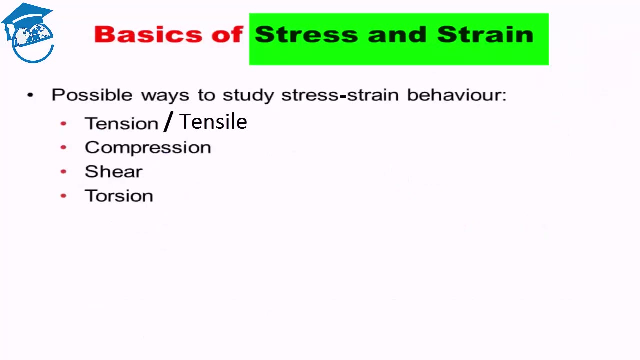 figures of stress and strain that you will see will encounter engineering stress and engineering strain Because they are much easier to handle And they kind of give you the basic idea of the material property. True stress and true strain are a bit complicated to denote. Fine, With this idea of stress and strain, let us see what are the different. 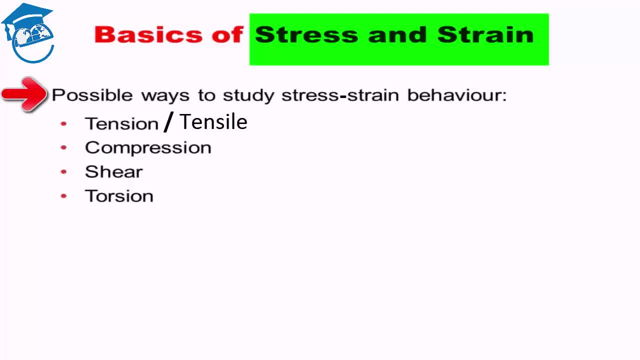 possible ways to study the stress and strain relationship, As I have said, that a stress, that is, application of a force, will lead to change in dimension, that is, it will produce strain. So under what conditions can this can be tested? This can be a tensile test. 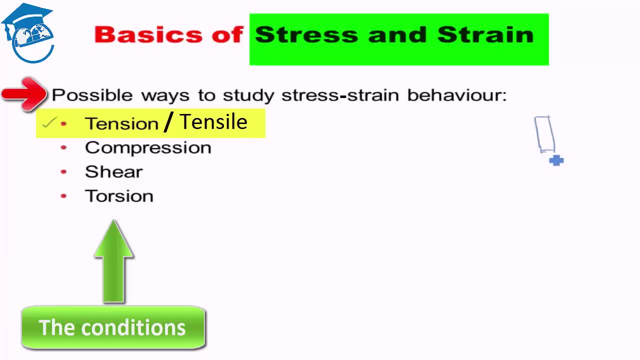 where, basically, you have a sample and tensile means you are trying to extend it, So this is tensile test. You can have a compression test. you have a sample and you are trying to compress it, So this is compression test, This is tensile. Then what you can have another. 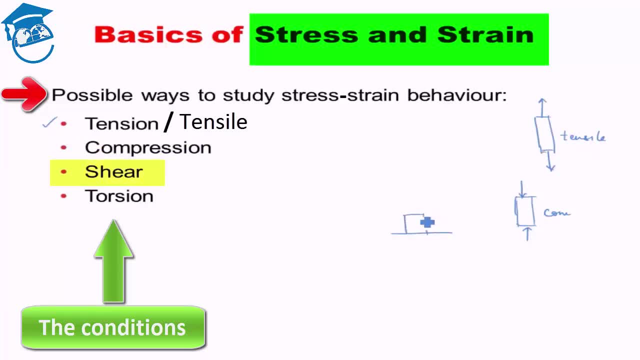 is: you can have a compression test. You can have a compression test and you can have a a shear. so you have a body and you try to shear it and that will have a stress strain behavior. so you can study stress strain behavior in tensile compression. 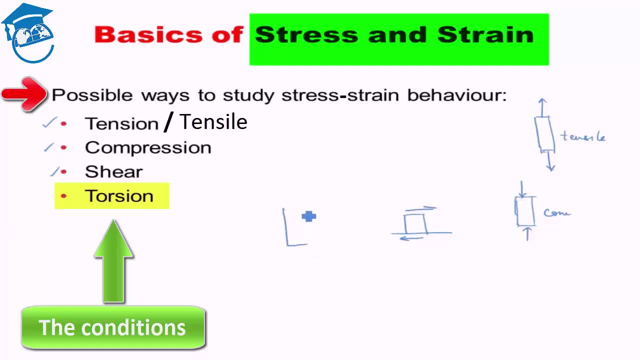 shear as well as in torsion. torsion is basically twisting the sample. you try to. you have a sample right and you try to twist it. you try to twist it and see how much twisting is possible for how much twisting force. so that gives you torsional test. but the most important type of stress strain test that will 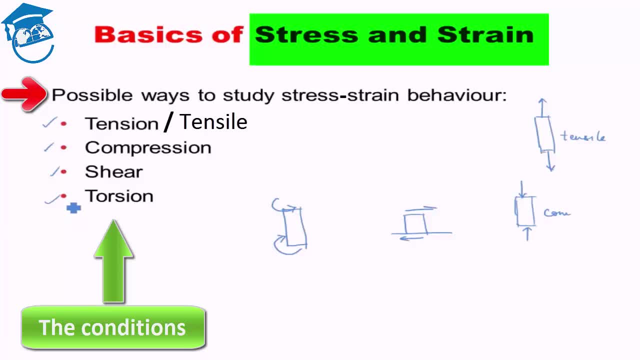 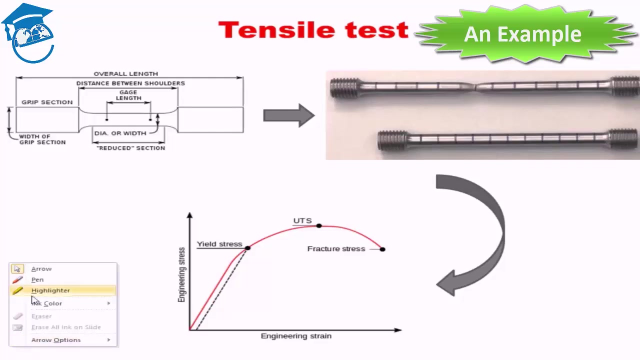 encounter, or the most practically applicable stress strain test that is used for the general mechanical property study. is that tensile kind? okay, so we'll from now on see the tensile test study. this is an example of tensile test. So in tensile test what you have is: this is a tensile specimen. 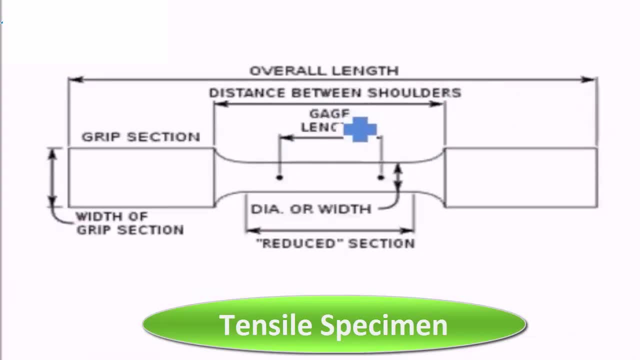 These are standard dimensions. I will not go into the standard dimensions. They are available in the standard dimension textbooks and therefore they do not add to the physical knowledge. So I will leave that aside, But I will discuss what are the different things. So this is my sample. It can either be flat or it can be rounded. The grip section can 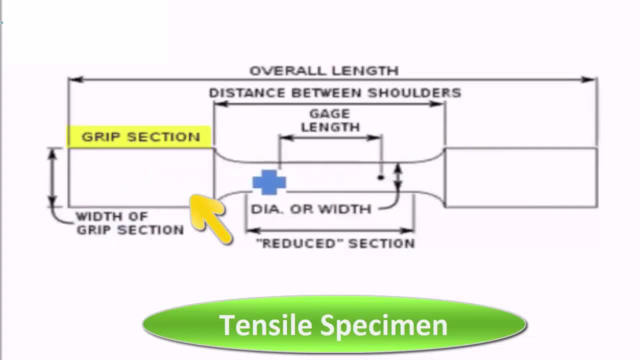 be rounded. If that is rounded, this is also rounded. If the thing is flat, then everything is flat. So basically, it can have a particular depth or it can be a radius. This is the overall length This region is basically put to grip. So basically, what happens? 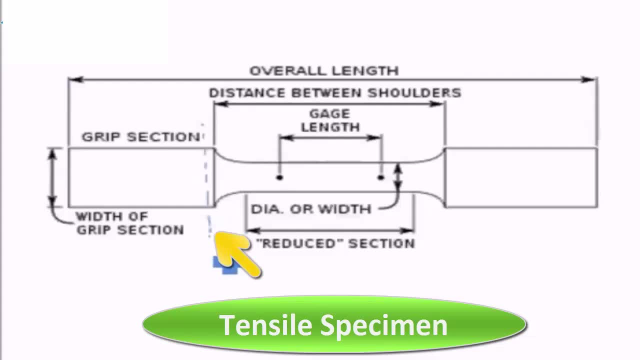 is, you have the tensile test machine, which will provide a grip here, It will hold here and here, and these grips, one will remain stationary and the other will be pulled. Okay, So this is the grip region. Then this region, actually this dot to this dot, is the. 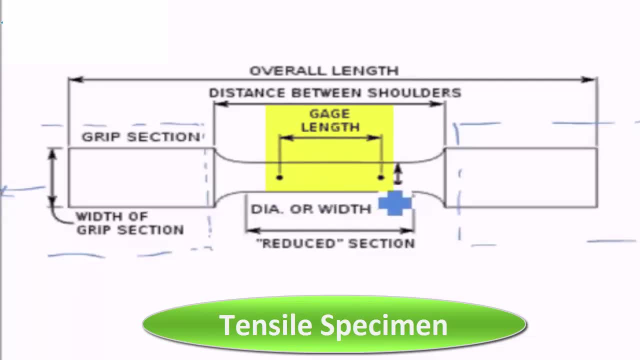 gauge length, and this gauge length is where the actual measurement is being done. Okay, So this initial gauge length is the L0 and we measure the change in this gauge length continuously during the tensile test is going on. So for any moment we have the stress measurement, how much load is applied, we know, therefore, 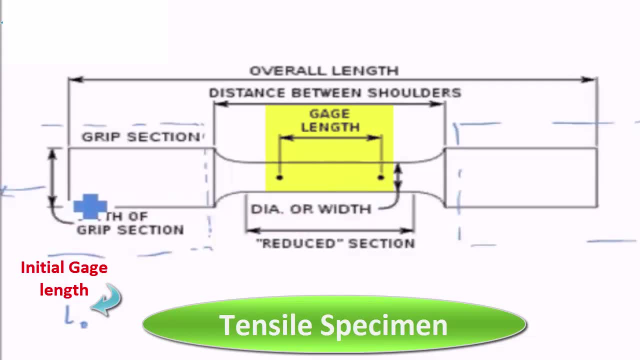 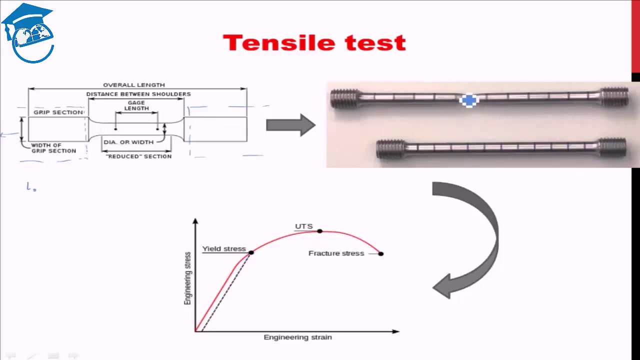 we have the stress measurement and against all the stress measurement, we have what is the instantaneous dimension at that moment. thereby we find out the strain. So if we take a sample- this was the initial sample which was put under tensile testing- and what happens, you can see, is that basically there has been a necking. this is known as